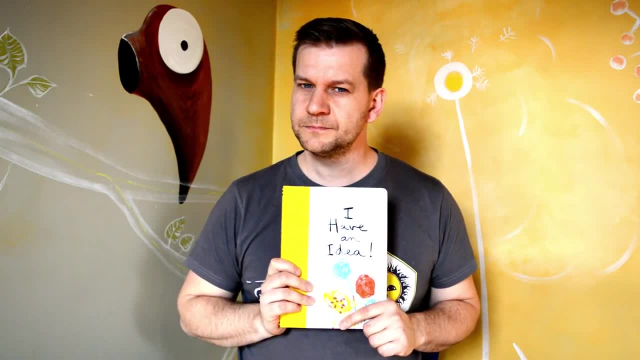 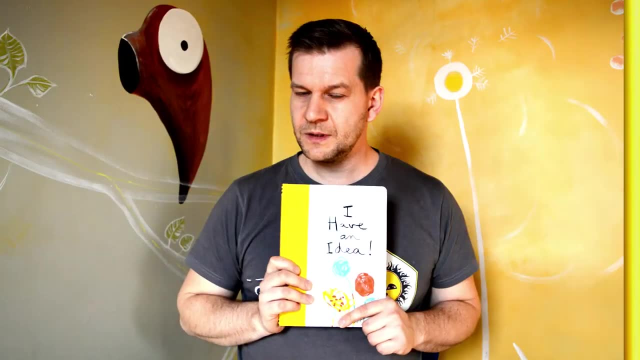 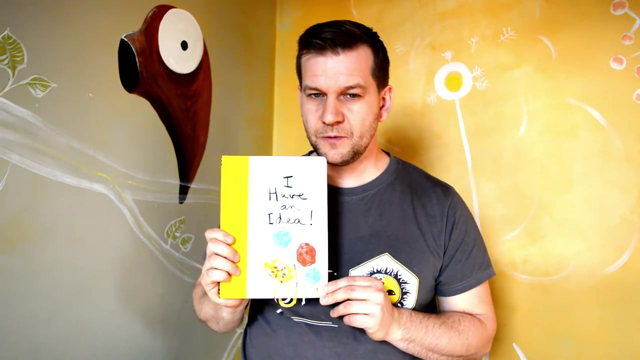 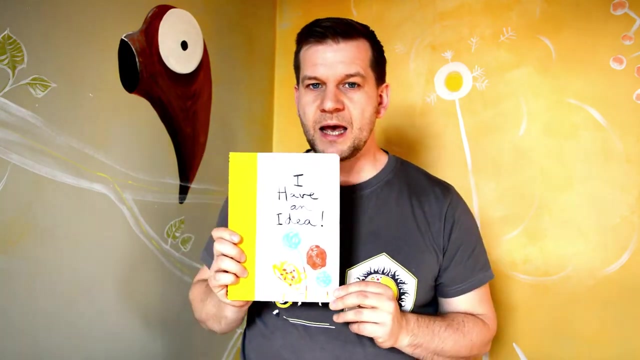 and think: what is my idea? Are you ready? So this book is all about ideas and it's about the process of how we come about ideas and what it could be. It's called Art. I have an idea by Henri Tulle and I'm gonna read it out to you, and then we're gonna have time for questions. 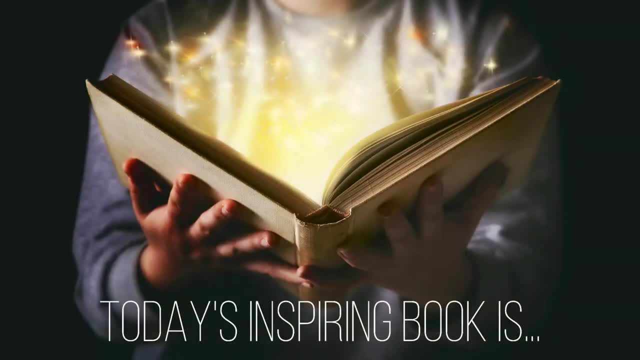 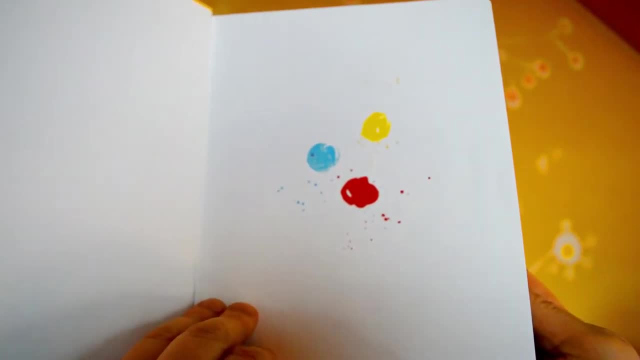 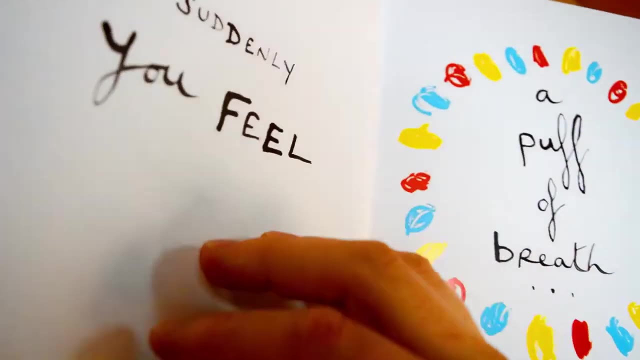 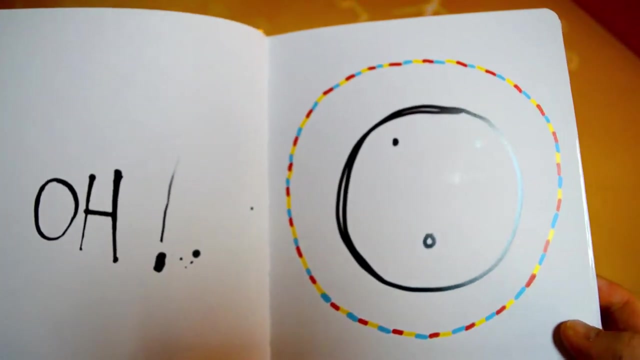 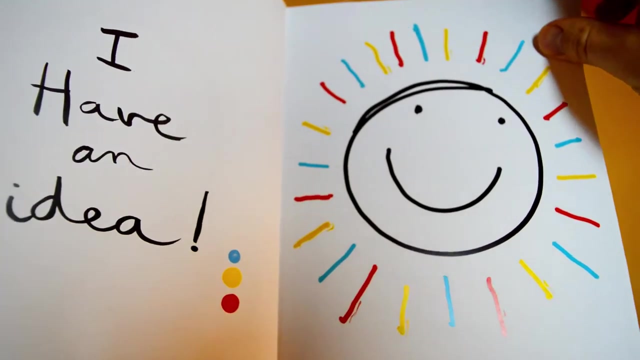 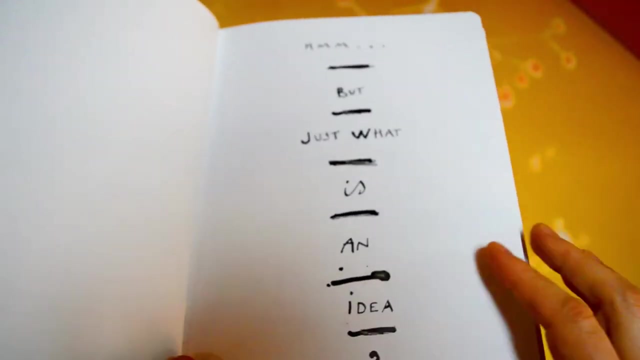 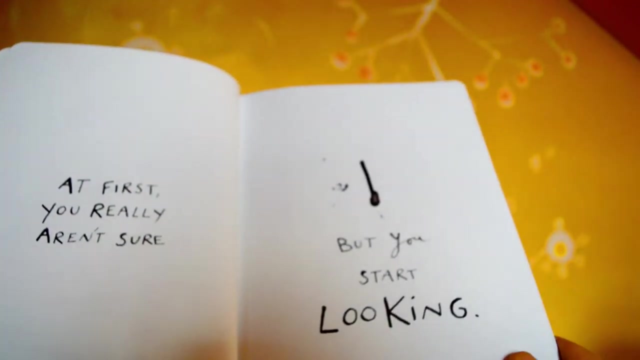 You ready? Today's inspiring book is I have an idea, by Henri Tulle. I always love that moment when suddenly you feel a pool of breath, I have an idea. It is a magnificent feeling. But just what is an idea? At first you really aren't sure, but you start looking. 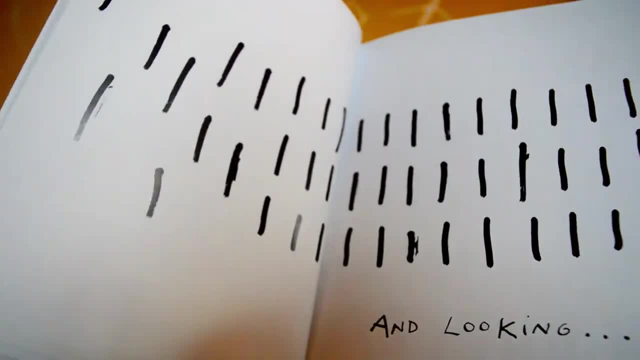 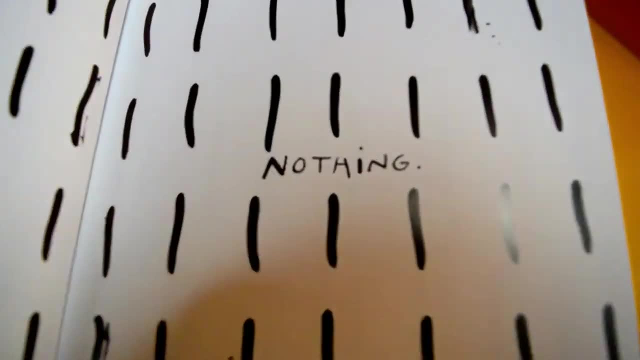 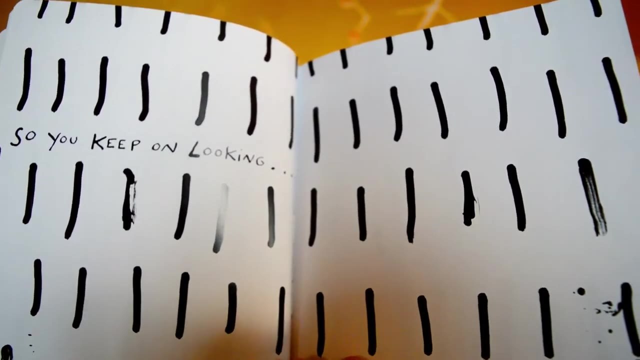 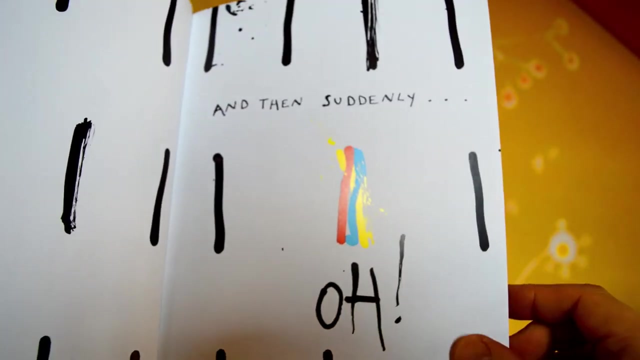 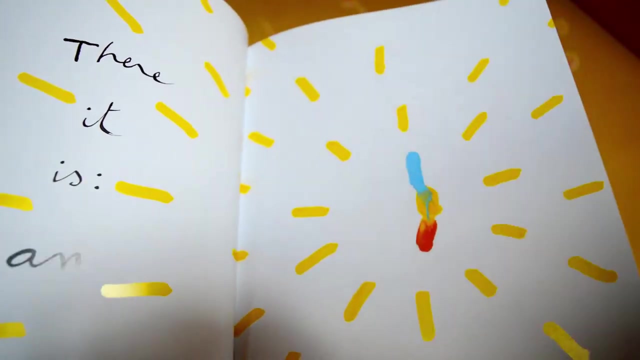 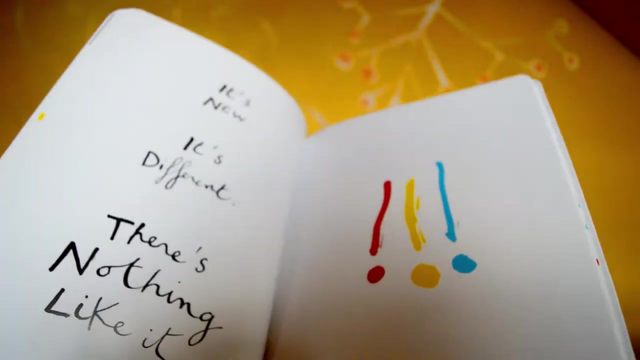 And looking, And looking Nothing. So you keep on looking Some more. It can get a bit boring And then suddenly, oh There it is An idea. It's new, It's different, There's nothing like it. 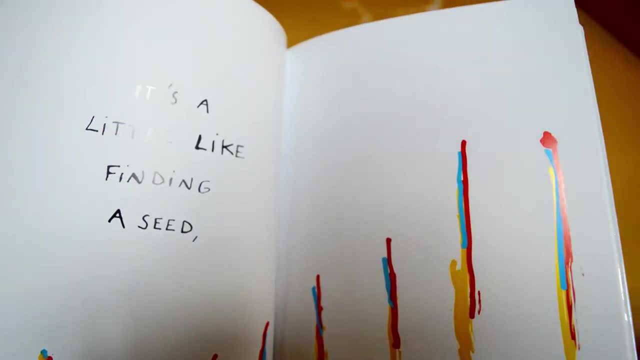 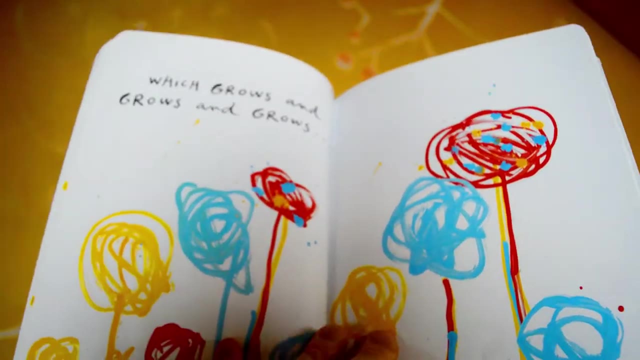 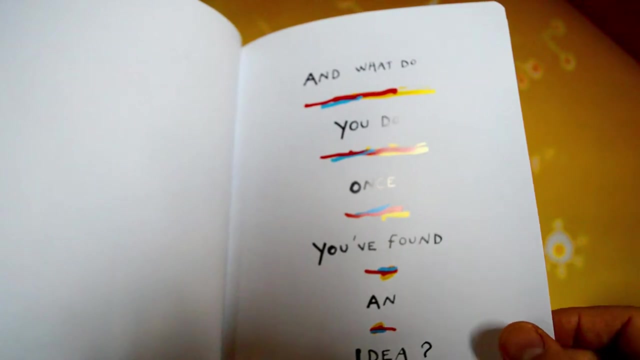 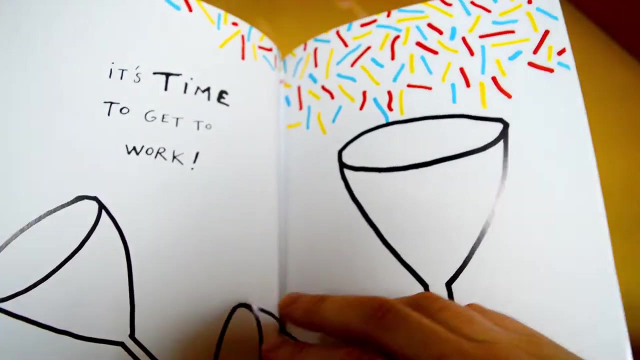 It's a little like finding a seed Which grows and grows, and grows. And what do you do once you've found an idea? Often ideas cause a lot of trouble. They can become rushing, They can be a bit messy And bubbly. 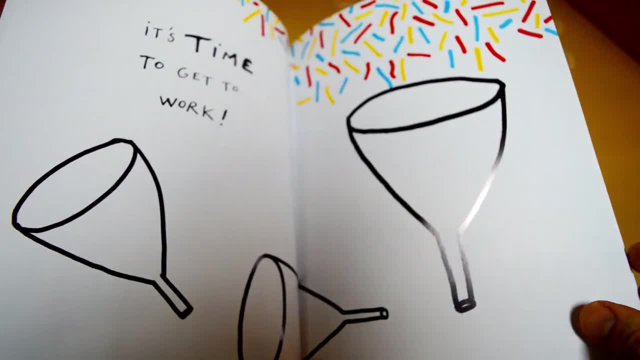 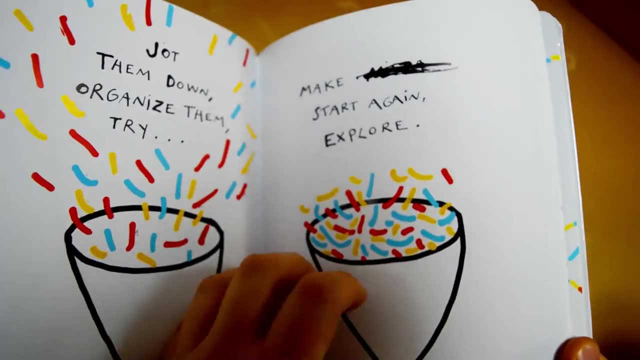 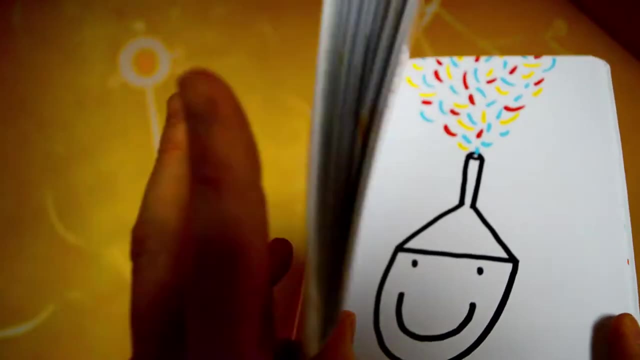 So it's time to get to work. Jot them down, Organize them, Try Make them start again, Explore, And right away you know it's good, because in every good idea there is a seed of something. So how do you feel? 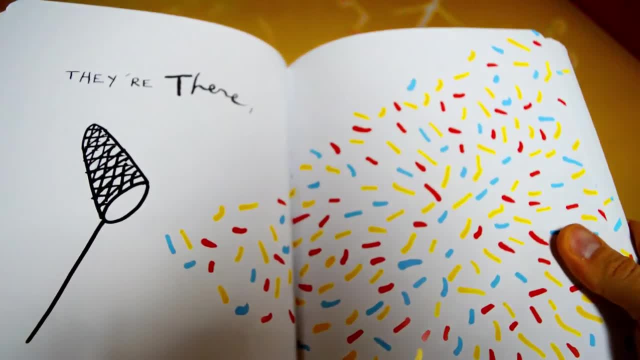 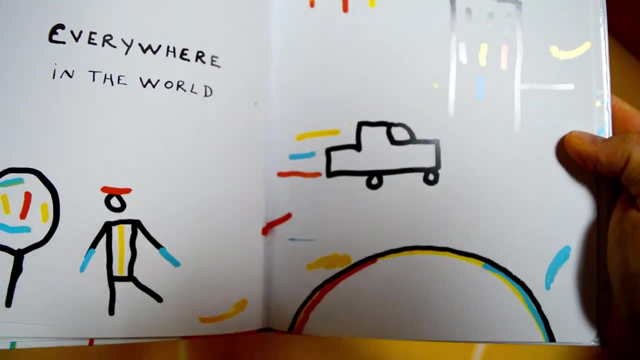 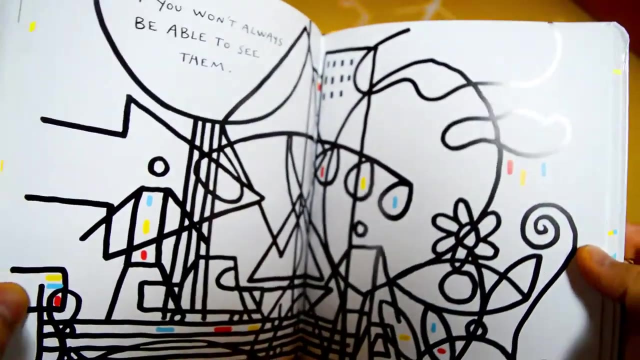 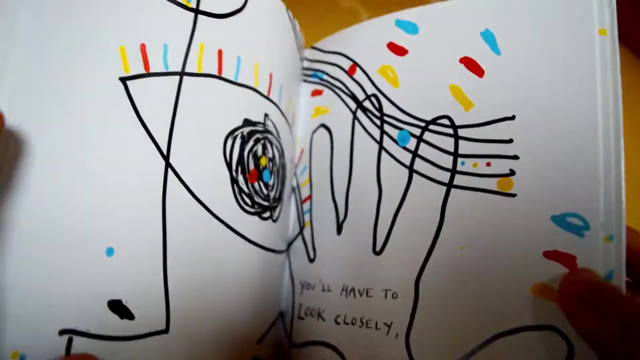 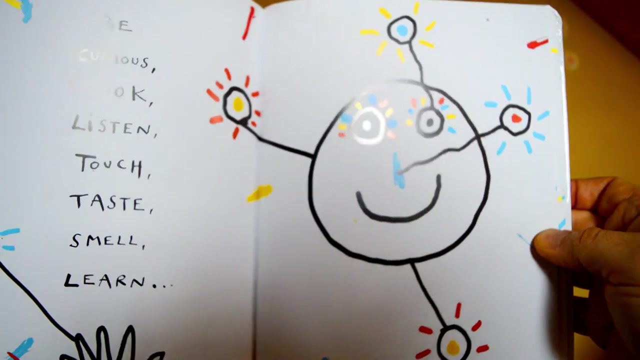 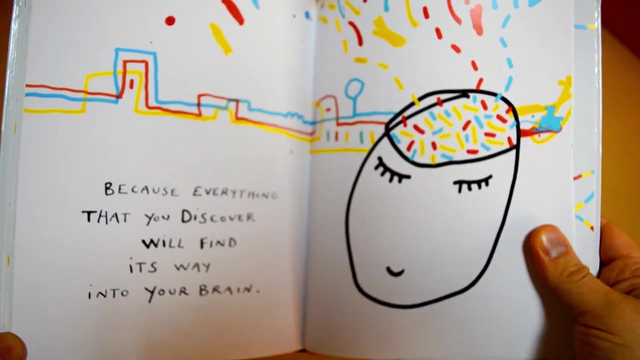 Find and cultivate those seeds. They're there Everywhere in the world, But you won't always be able to see them. You'll have to look closely, Be curious, Look, Listen, Touch, Taste, Smell, Learn, Because everything that you discover will find its way into your brain. 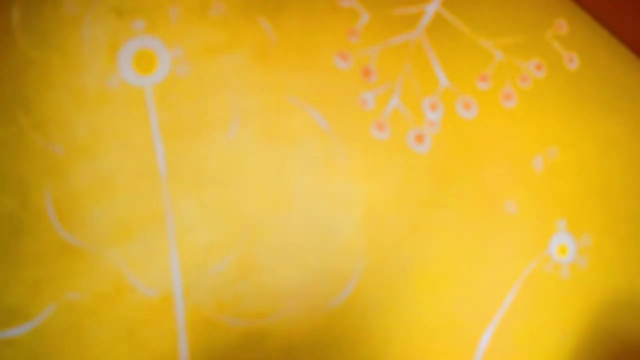 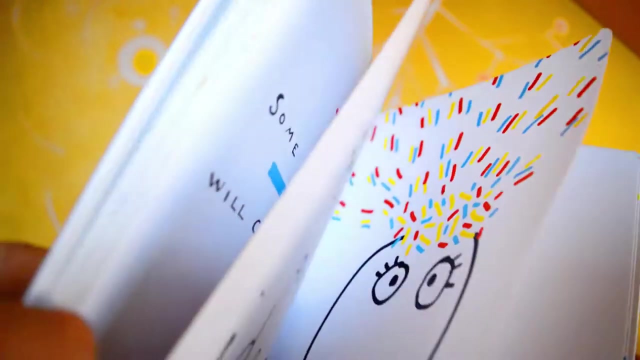 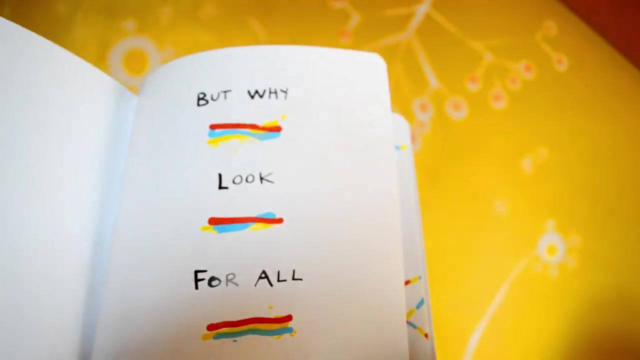 And then one day, while you're still looking, Some of the seeds will cluster together, And then, Oh, I have an idea, An idea. But why look for all those ideas? Maybe just for the fun of it, Maybe to change the world? 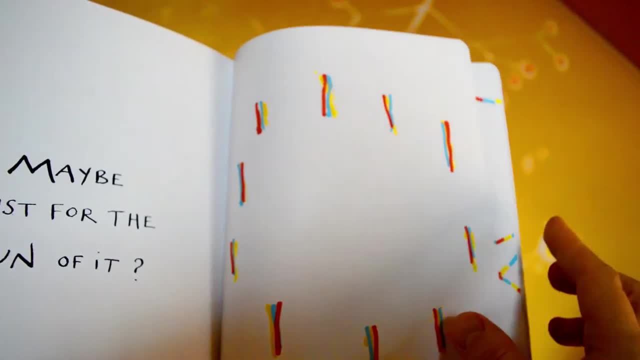 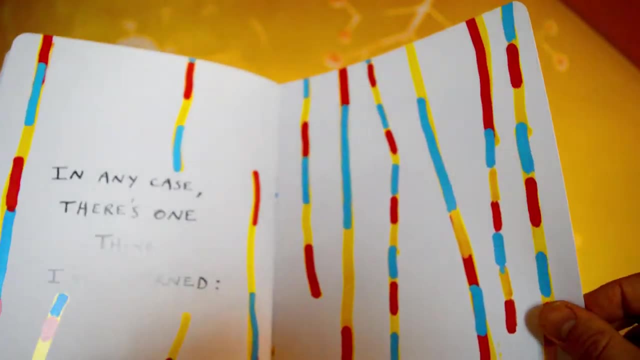 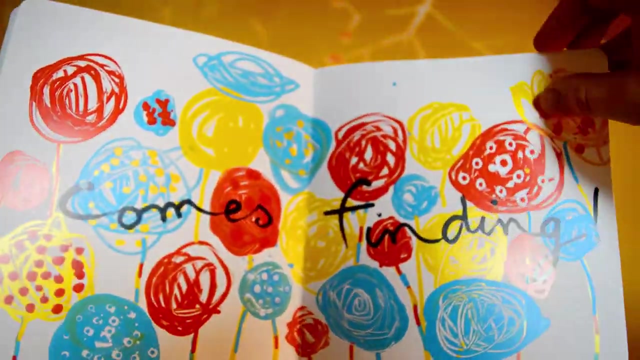 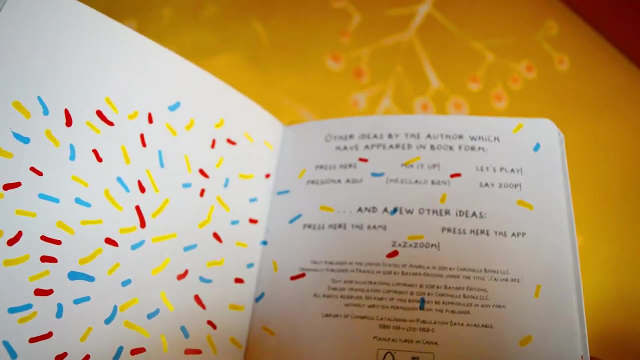 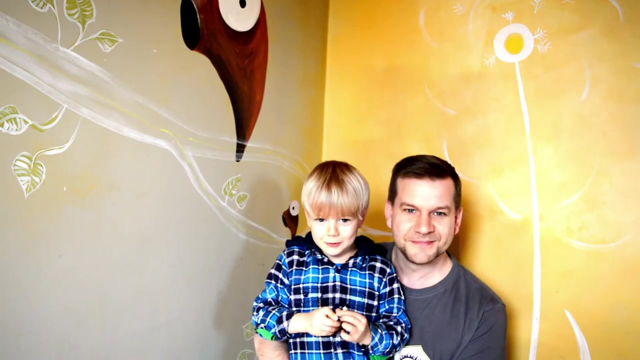 In any case, There's one thing I've learned: With looking Comes Finding, And so If you look, You To Find Your. And now it's time For what? For the questions. So The questions I have for you. 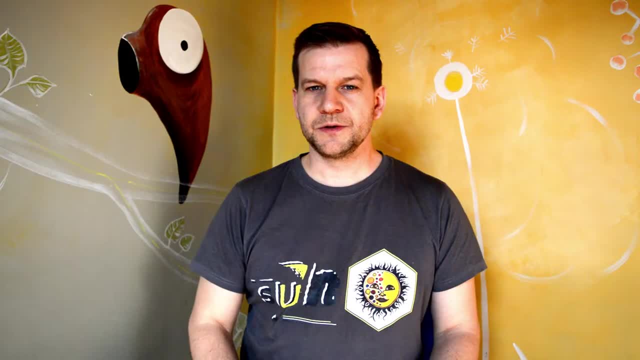 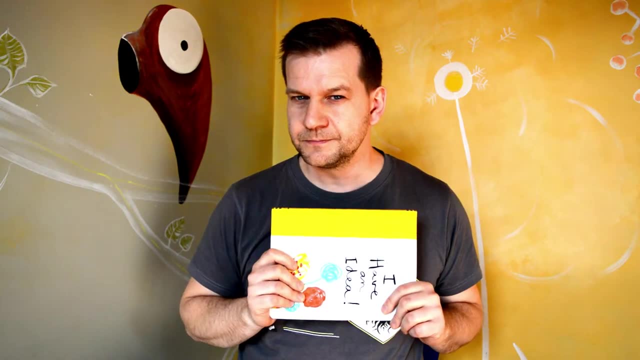 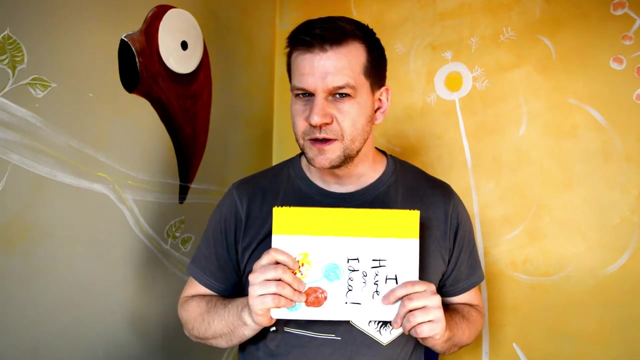 Is: What's your one big idea That could change the world, And Not only that. You have to explain Why Would this idea change the world? So What's your big idea? To help you do that, You can take something to draw. 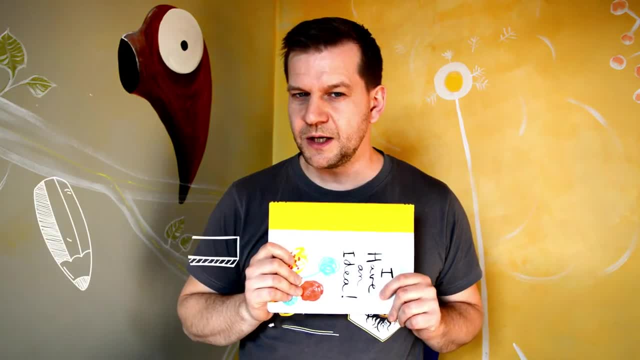 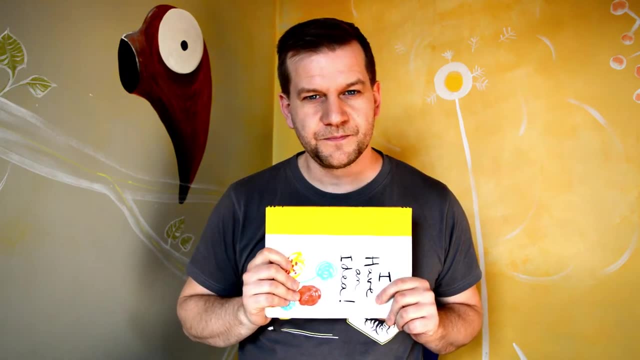 And draw it first As a picture, Or if you can write, You can write it And get your parents and your family to do the same And tell their ideas And explain why. Good luck. So If you like this video, 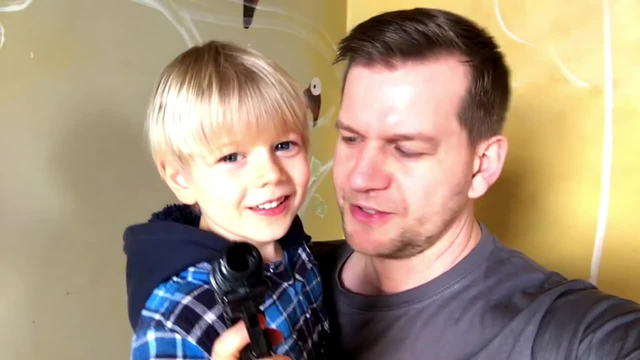 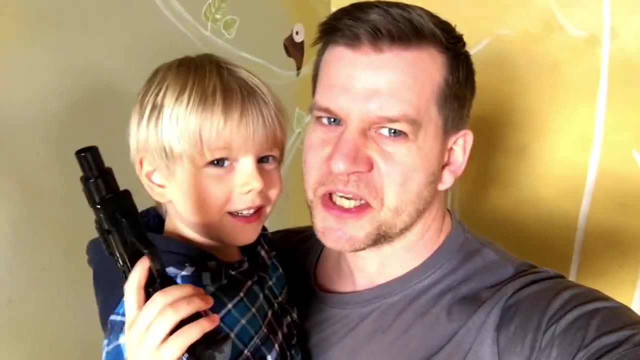 Please share it And subscribe, Like it And then comment In the comment section So we can learn about your ideas. Get crazy.